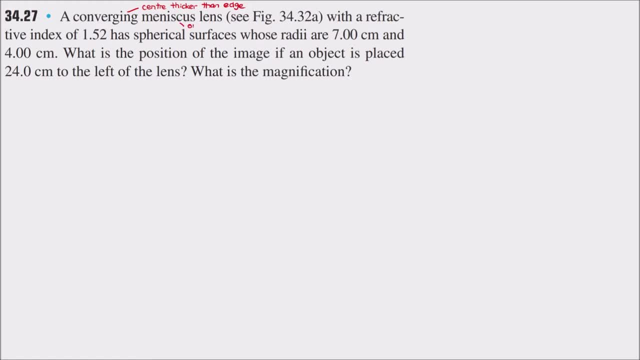 So meniscus lens tells you that one side will be convex, one side will be concave. Then they tell you the refractive index is 1.. So if you say it's 1.52, that will be our end of our lens material. 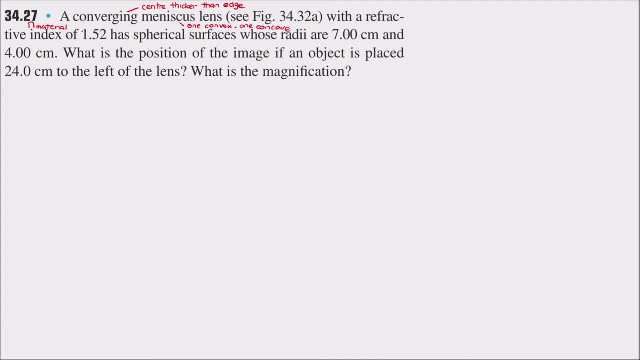 So they tell you the spherical surface. both of them will be 7cm and 4cm. So 7cm and 4cm here will be R1 and R2.. You don't know which one is R1,, you don't know which one is R2.. 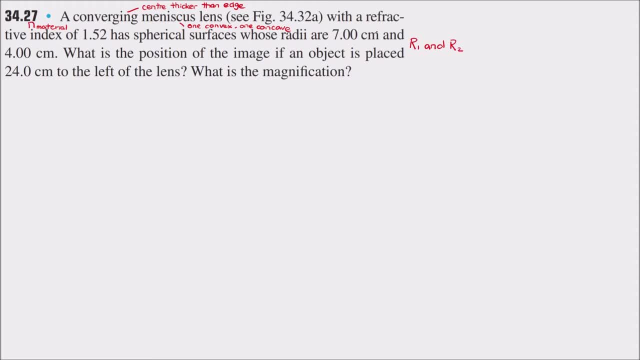 And it's important to find out which 7cm belongs to R1 or R2.. So now we are going to investigate: what should we put for R1,, what should we put for R2.. And besides investigating, we also need to know what are the signs that we need to put to determine the focal length. 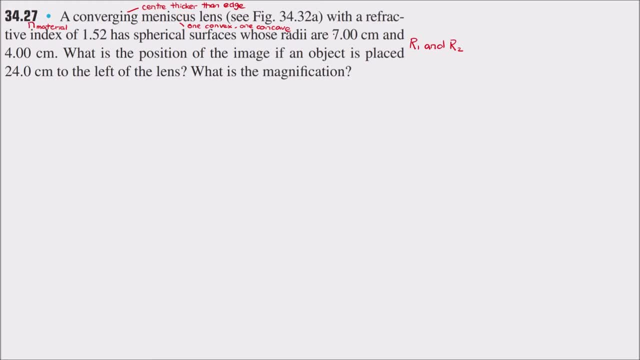 So let's give it a try. Converging meniscus lens. How do you create a converging meniscus lens? You can create it by using a sphere of 4cm- this green sphere here- And a sphere of 7cm as its radius. 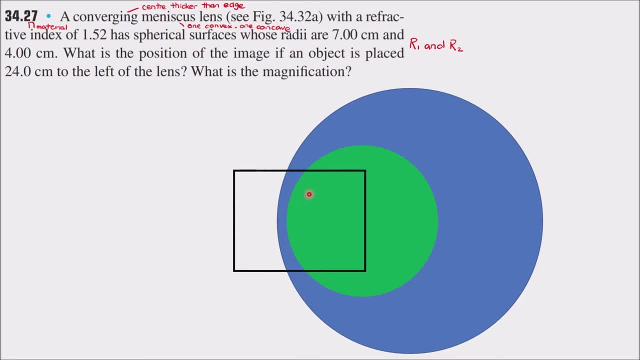 And then you can create a big sphere over here, And if you overlap it in a way that the larger sphere is in front, the smaller sphere is slightly behind, Then you can see that this blue portion here will essentially be a meniscus lens. 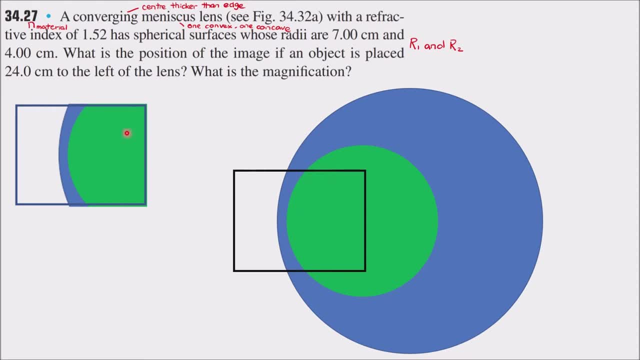 So let's snip it out, the meniscus lens that we have, And you can see from this meniscus lens that the edge here will be thicker compared to the center. So in this case, So in this case, So in this case, 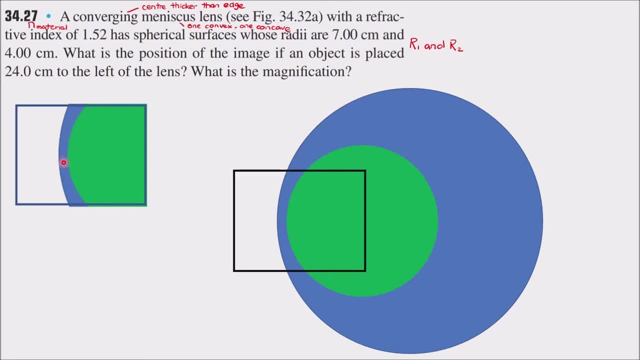 diverging meniscus lens because it has a center portion which is thinner than the edge itself. so we, we don't want this meniscus lens, we want the opposite of it. we want a converging meniscus lens. so what we do? we should change the order of the circles. so now we bring the circle which has a 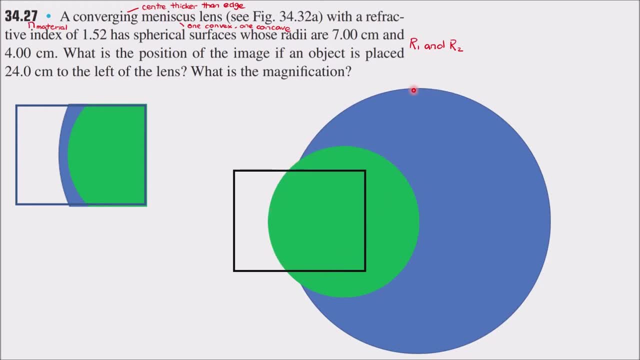 radii of 4 cm in front and put this large sphere over here slightly behind and if we invert the order, bring the blue circle to the front. then we see that this green green color portion here is essentially just another meniscus lens. if you snip it out you see that the center portion over 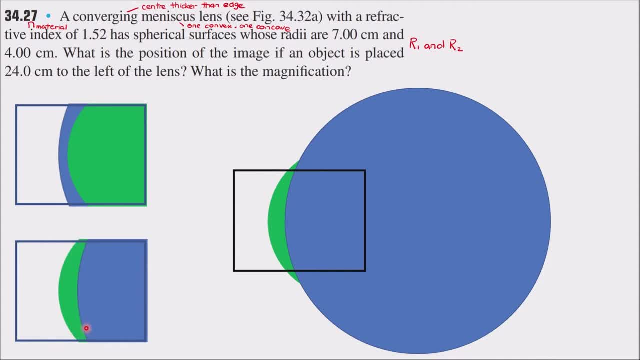 here is thicker compared to the edge over here. so this is what we are looking for, because we are looking for converging, then we say the center must be thicker than the edge. so this second diagram here is a much better representation of the maniscus lens that we want to find. 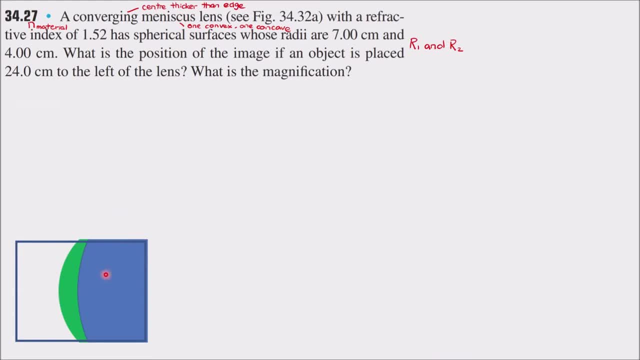 so, yep, that's what we get. so let's draw this diagram here, so we know that this green circle here is the smaller circle. therefore, here should be R1. this R1 there should be equal to All cm, because green circle is a small circle from just now, right, so it should be 0.040 meter, whereas for r2 over. 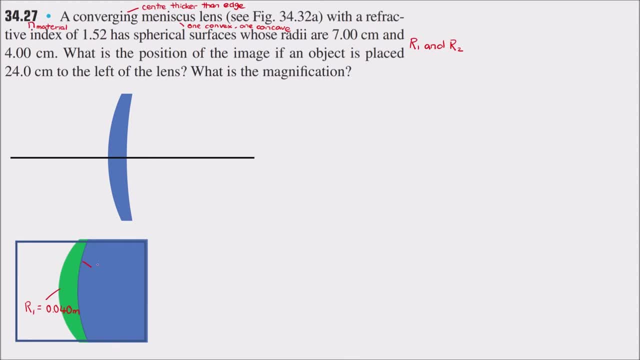 here it's made of a larger circle, so larger circle should have a larger radius, so r2 should be equals to 0.070 meter. okay, but it's not just not that simple, okay, you still have to determine whether the sign is correct or not, okay, so let's try and determine the sign so you have like for this first. 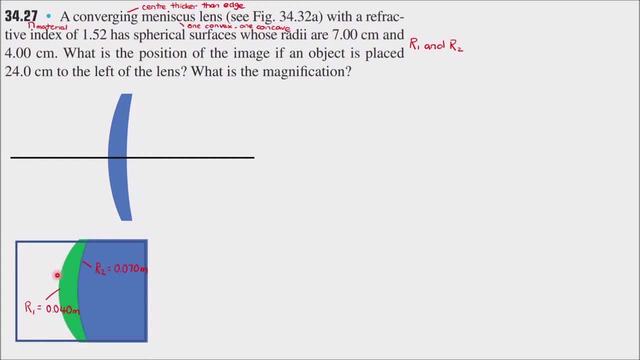 surface over here. your refracted ray will be inside the lens you incident here, then you get reflected over here. so the ref, the reflected rays, on the right hand side of the first surface. how about the sandor curvature? it's also on the right hand side of the surface. 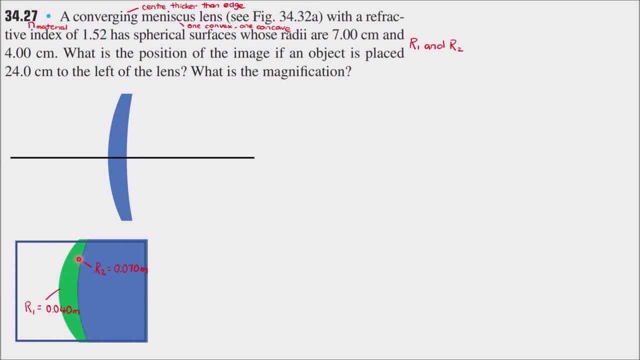 therefore, since they are on the same side of the surface, both on the right hand side of the first surface, you get a positive value for r1. okay, positive. how about r2, r2- you will have your ray, reflected ray, coming out from here. okay, the refractory will come out from. 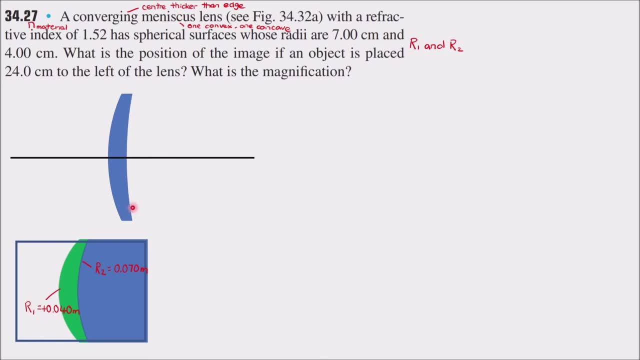 here. so you know that refractory is on the right hand side, or of the second surface over here. how about the center of curvature? the center curvature will also be on the right hand side, because if you trace our circle, the circle will be around here. so center is on the right hand. 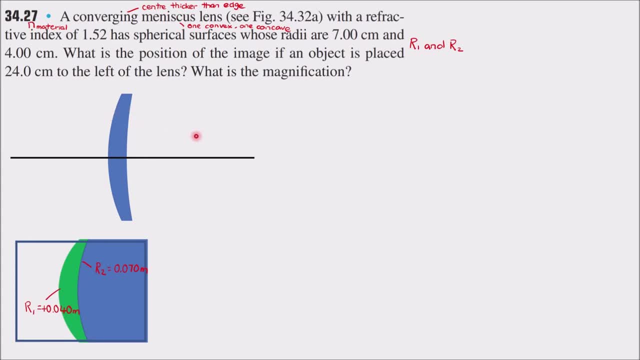 side of the second surface. the refracted ray is also on the second. it's on the right hand side of the second surface. therefore, they're on the same side. therefore, we know that r2 here should also be positive. r2 here is also a positive value. okay, so now we know r1 and r2, and let's 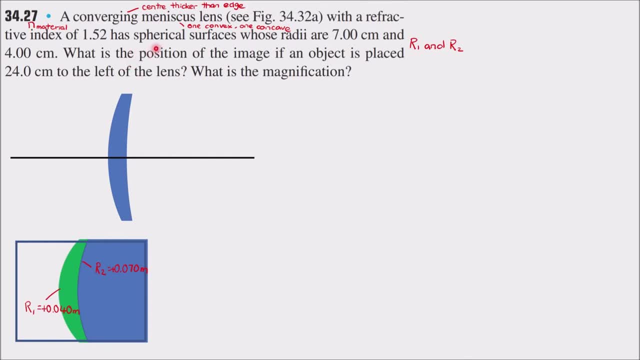 look at what the question asks for. the question asks: what is the position of the image if an object is placed 24 cm to the left of the lens? so let's put it down: our object. okay, object is 24 cm to the left of the lens. let's say: here is where our object be. 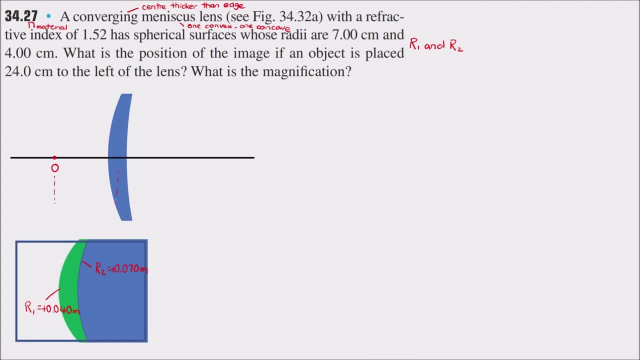 then if you measure the distance to the center of the lens, you'll find that this distance here should be 0.240 meter. okay, so how do we determine the position of the image? well, uh, if you want to determine the position of the image, you have the object distance. what you 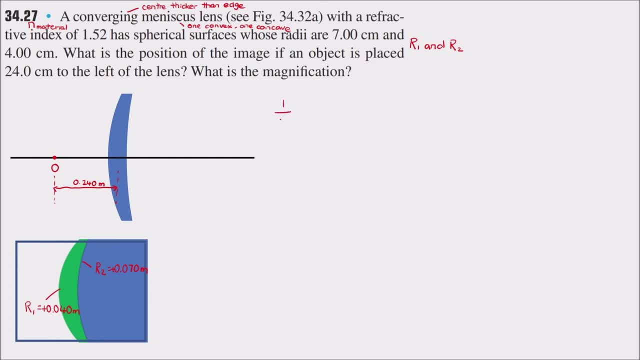 have is a equation called the thin lens equation. then you can relate the object distance, which is what you have, 0.240 meter- with the image position, which is image distance, what we can find. but we need to know first what is the focal length for this meniscus lens over here. therefore, f is a. 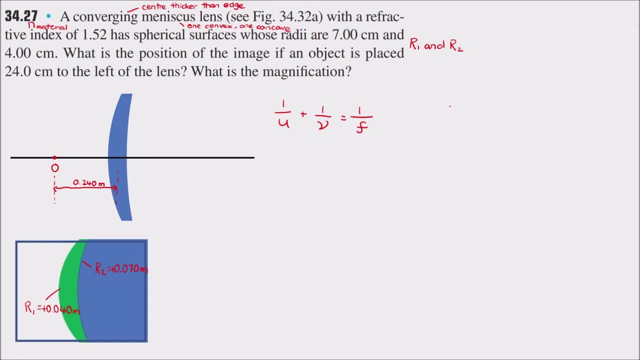 thing that we don't know and we need to determine the focal length using the lens maker. equation over f equals to the refractive index of the material divided by the refractive index of the medium minus one. then close the bracket for the first component. second component will be one over. 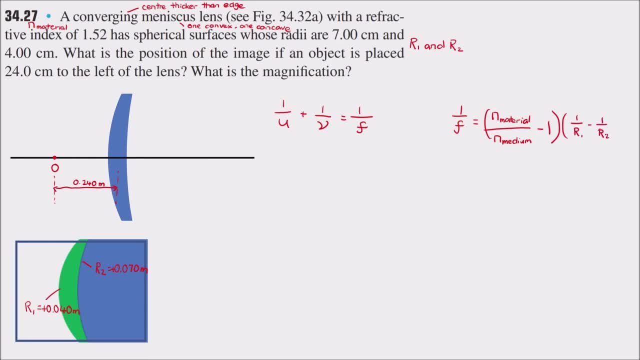 r1 minus one over r2. okay, so it's a matter of substitution. you know that the lens material is having a refractive index of 1.52 and they didn't mention what is the surrounding medium. if it didn't mention, you assume it's a vacuum or it's just air which has a refractive index of 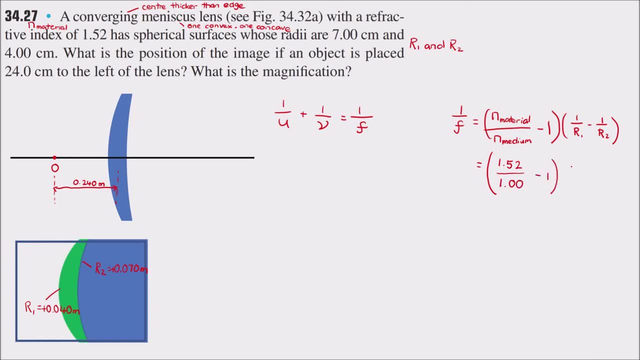 1.00 minus one. okay, then you have one over r1. r1 is positive 0.040. then you have your r2, which is also positive 0.070 meter. okay. so if you do your calculation for everything, you'll find that the focal length will be equals to 0.179 meter. okay, so, 0.179 meter. 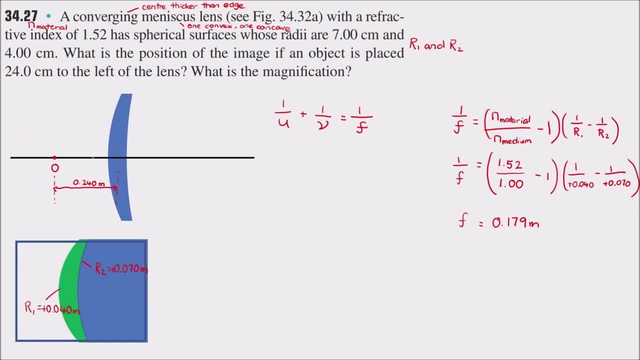 if you plot it back onto this, uh, this diagram over here, it will be somewhere around here, maybe, okay. so we have cleared up this part and let me label the distance. distance from the center should be equals to 0.179. okay, now we have done this part, let's get back to the thin lens equation over here. okay, we know u, we. 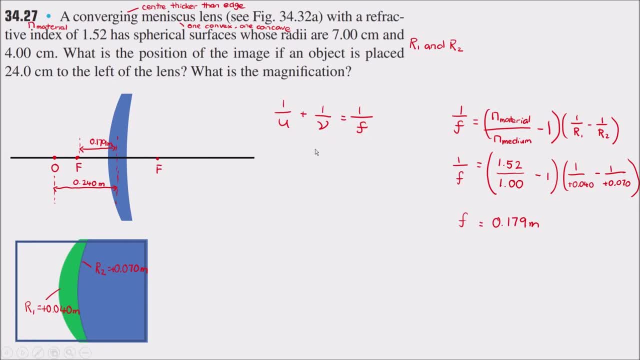 know f, and now it's just a matter of substitution. one over u. we know that is uh. okay, if you want to determine the sign of u, remember that if the object is on the same side as the incident rate, then it's positive. opposite side to the incident rate and it's negative. okay, so from here you can. 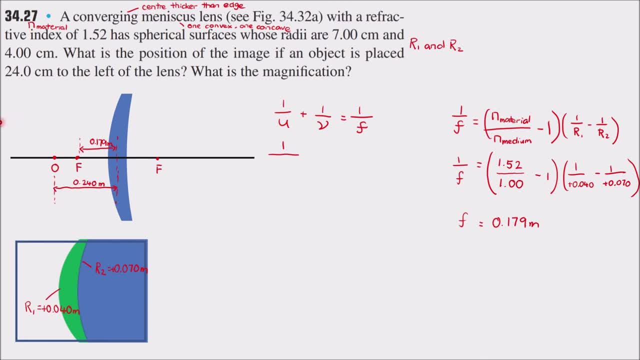 see, the object is still in front of a lens, then the incident rate is also in front of a lens. so if the incident rate and the ray and the object is both on the same side of the lens, you know that u here should be a positive value. okay, so it should be positive 0.240 then plus 1 over v. 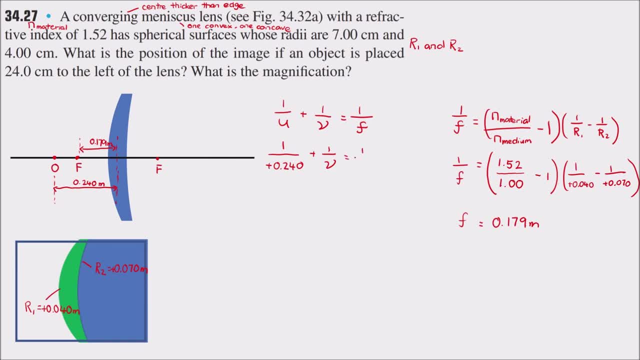 things you want to want to calculate, then equals to 1 over f for the f here the f is equal to 1 over f is 0.179. so this should be a positive value. so let's double check whether positive should be the right answer. well, it mentioned that it's a converging lens. converging lens is a positive. 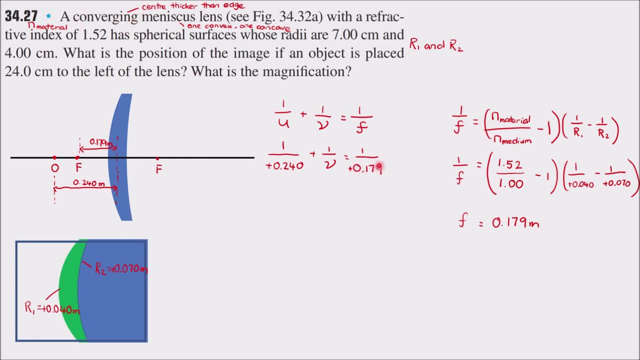 lens, so you should get positive focal length, which is true over here. okay, so now, if you do our calculation, we will find that v will be equal to 0.712 meter, and it's a positive value. if it's a positive value, what does it tell us? is the image should be formed on the same side. 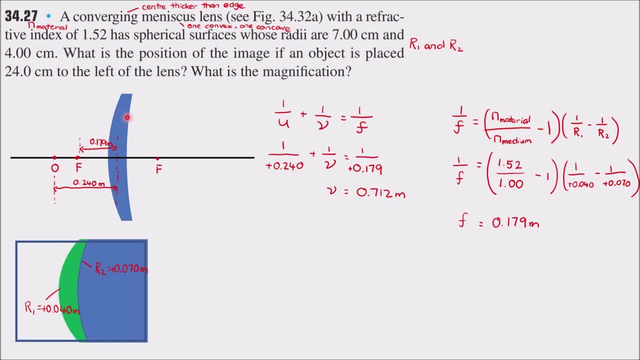 as the refracted ray. so the refracted ray is coming out of the lens over here and on the right hand side of the lens. so our image should also form on the same side as the refracted ray. so the image should be formed on the right hand side. therefore, if you try to plot it over here, 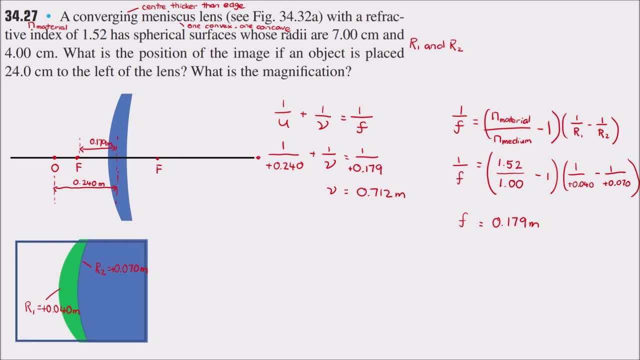 it's quite fast away, somewhere over here, probably even further away, so this is where your image will form, okay, so if you want to really put it in words, then you can say: this is 0.712 meter to the right of the lens, okay, so, okay, the next question: what is the magnification? 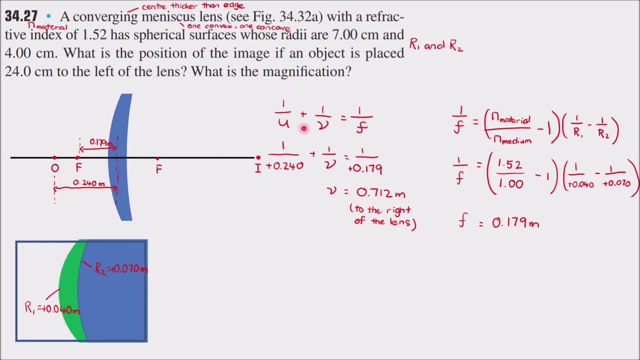 well, we know v, we know u. now it's just a matter of substitution. we know that m is equals to negative v divided by u. so the image distance is 0.712, a positive value. the value is 0.712. the distance is 0.712. the distance is negative. the value is 0.712, a positive value: the. 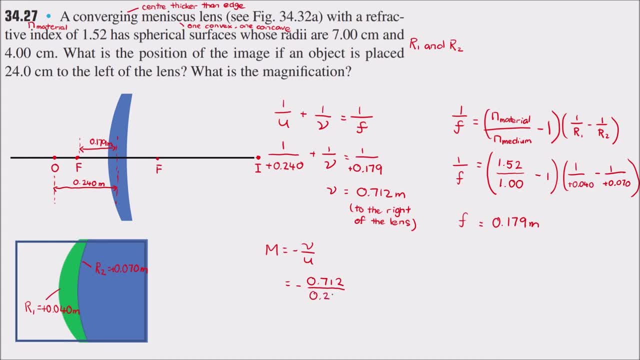 u here should also be a positive value: 0.240. so if you calculate these two things, you should get an answer of 2.97. and remember, it's a negative value, okay. so what does it mean over here if it's a negative value? if it's a negative value, it tells you that this- um, this is an inverted image, okay. 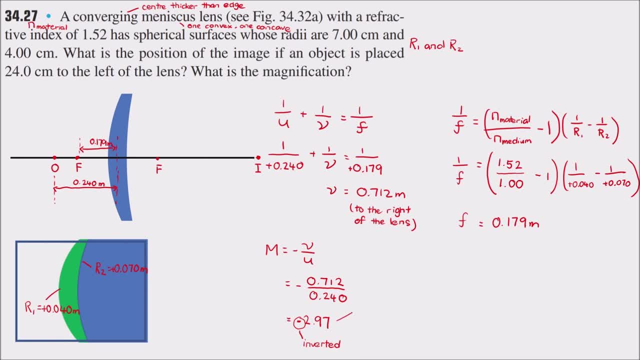 what else does it tell you? if it's larger than one, then it's magnified. okay, so combined with v is equal to 0.712. we know that the image should be formed on the same side as the refracted ray, so the image is formed by the intersection of the actual refracted ray that we have. it's no. 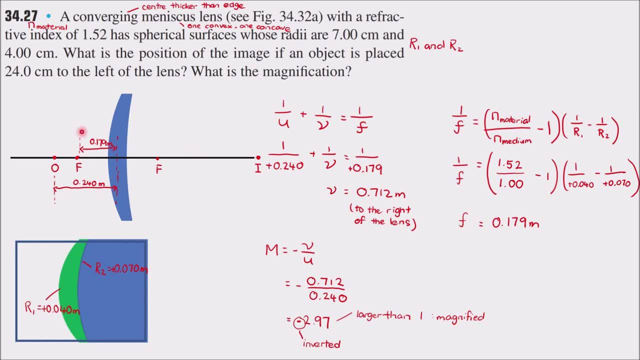 it's not the extension of the refractory backwards. if it's extension, then the image should be formed on the opposite side to the refractory, but now it's on the same side. we know that this image here is formed by intersection of the actual refractory itself.